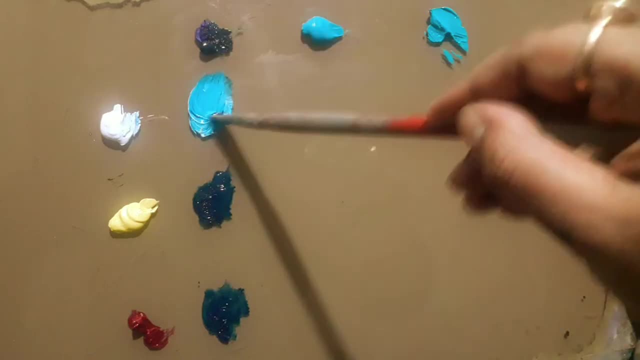 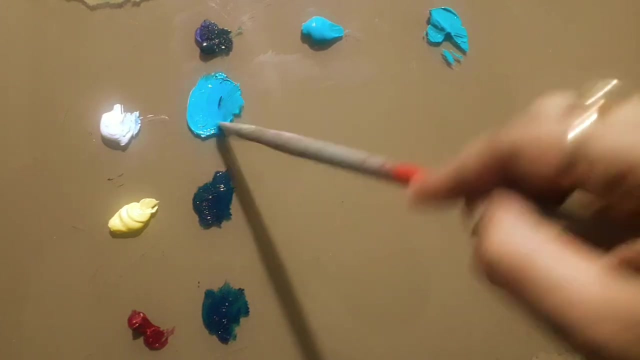 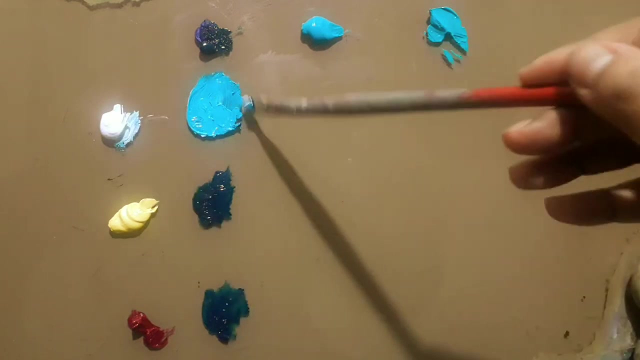 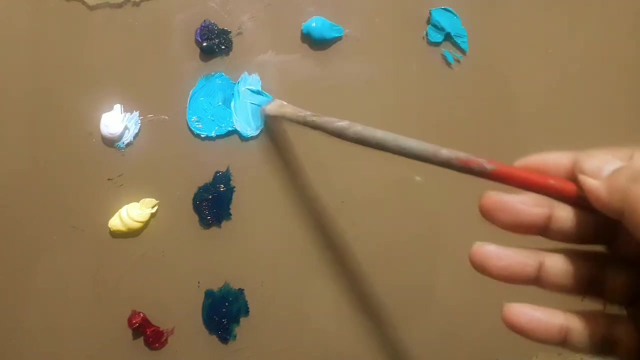 Looks pretty similar. Yeah, it's exactly the same value that I've acquired. It's getting a little darker And I'm going to add a little bit of a blue. Let's add white to this so that we can compare these that are lighter value colors and we. 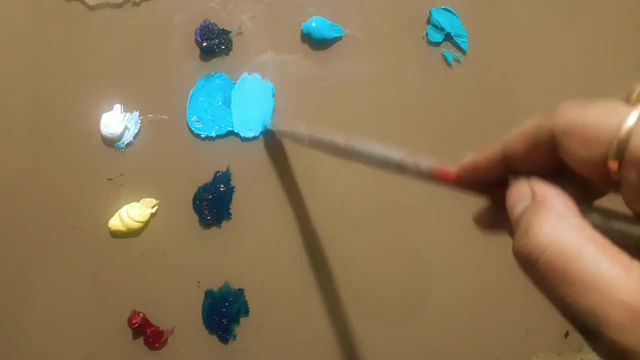 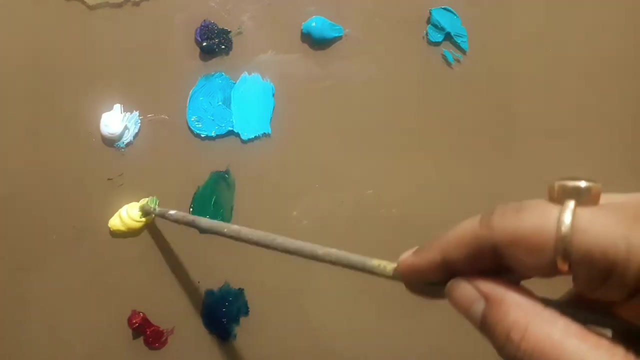 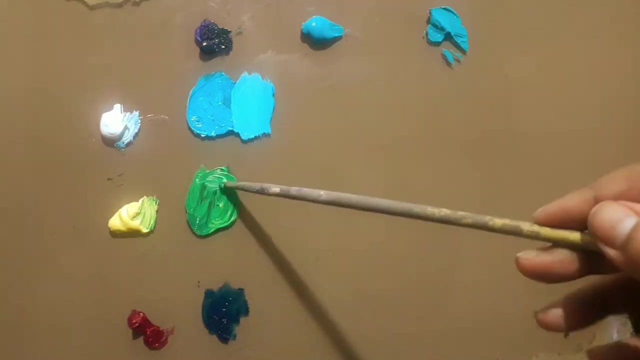 get to know what happens when we mix them with white. Now let's mix this with yellow. This is not a very bright yellow, but still it'll do its job, because this is lemony. This is not as powerful as cadmium. 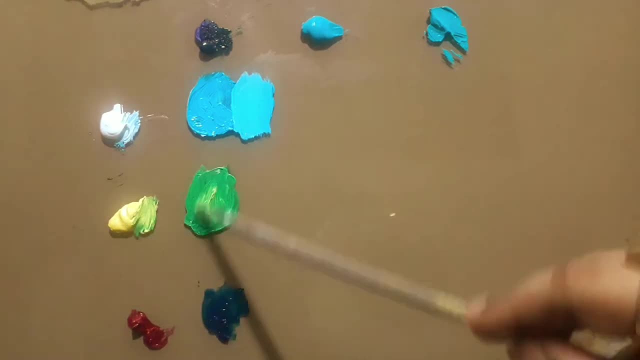 But let's take it to the limit. And as we can see, the cyan itself, phthalo blue and phthalo green- both are producing a very bright green color, And here we are going to mix a little bit of magenta with this color, this mix. 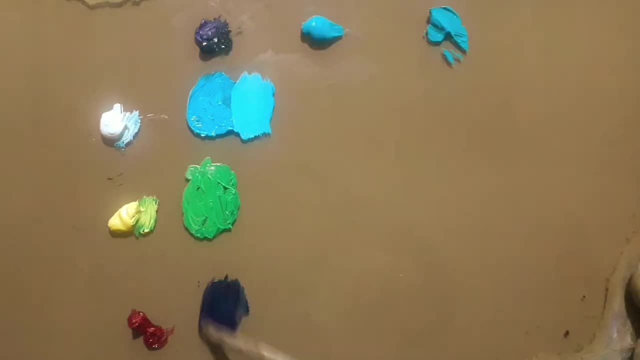 So we're going to mix this with a little bit of magenta. Let's see if we can mix a little bit more And we can mix a blue color. I think it'll be easier because we already have phthalo blue here. 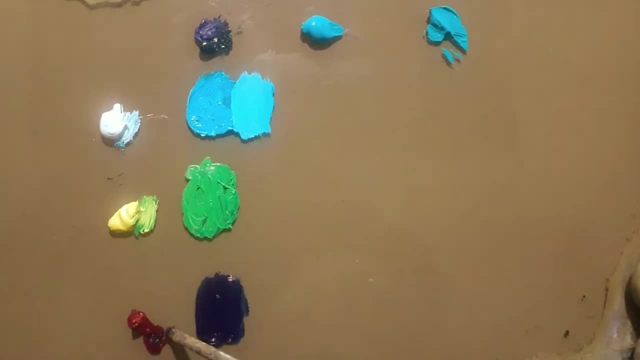 And it'll be important to mix a little bit of white here so that we get to know about the nature of the color. I'm mixing a little green so that it doesn't get too much purpley bias. Let's add a little bit of white. 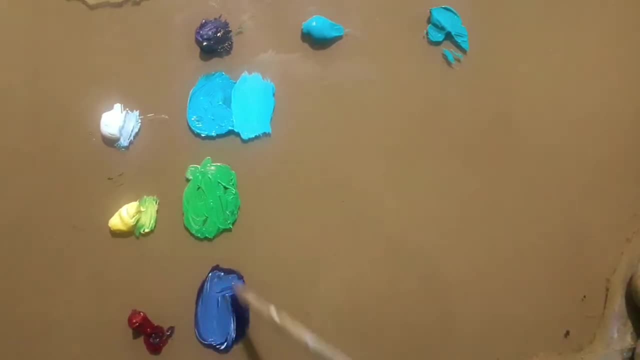 It already has got a cyan in it, So this is becoming a bit more violet-y. This is already very deep blue. This may not be a blue like that, but this is a blue. no doubt Let's add a little bit of green. 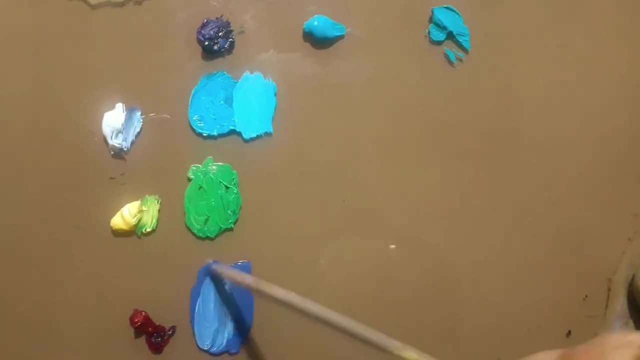 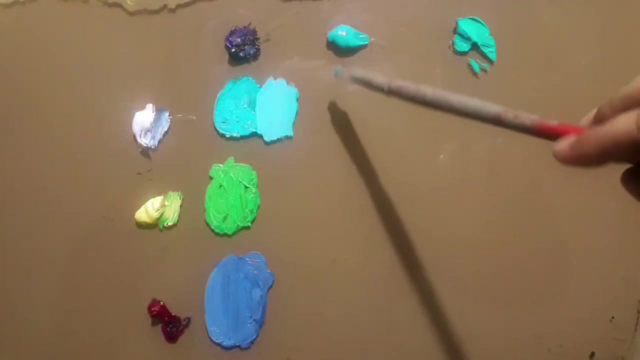 And let's see what happens there- And add a little bit of white. This is a nice blue color, slightly muted, Yeah. Okay, so moving forward with the proprietary one. And this doesn't contain any cobalt teal. This is mostly this mixture with possibly white. 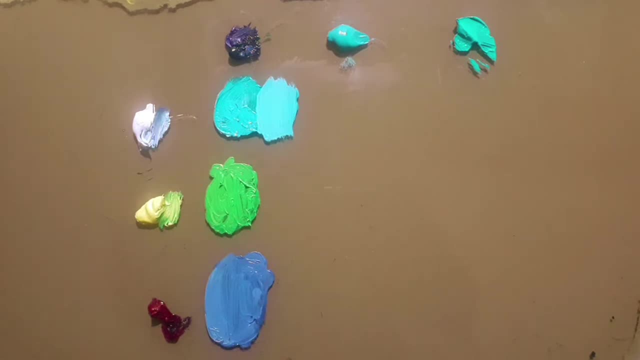 And that's why it produces a slight amount of dull results, But this still does the job, as, although this is appearing slightly duller in front of the real cobalt teal, but this is still a very bright color. So let's just use this on its own, just the way we have used that one. 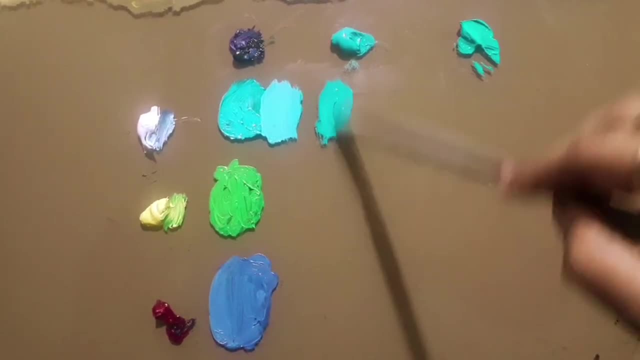 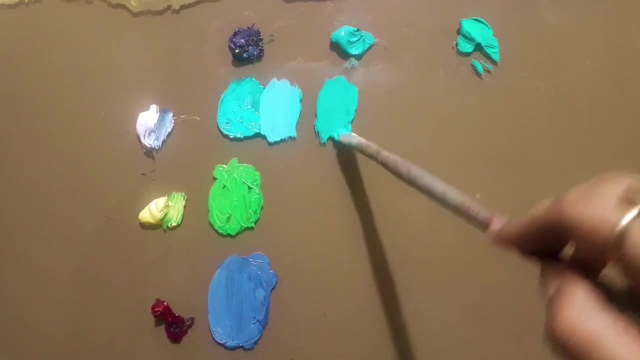 Let's just add a little bit of oil here, Let's just get to that creaminess of this particular paint. So this is Thelomade, But there is no problem, This is still a very bright color And if you want to use this sort of an effect, so this is a very good alternative. 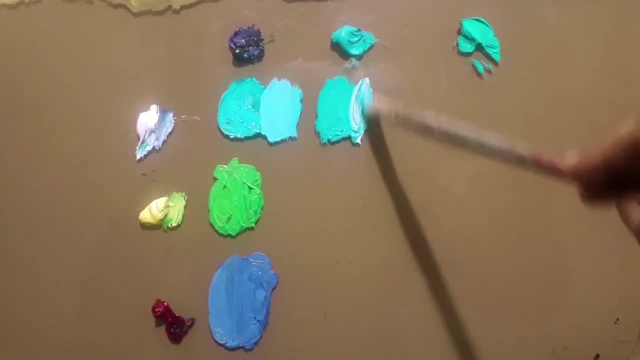 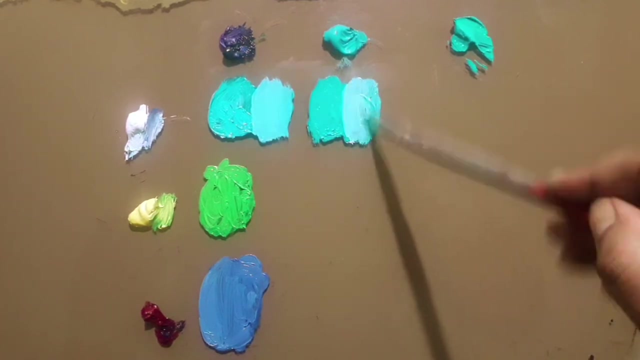 To this, which is humongously expensive. So let's just add a little bit of white And let's see if it comes anything closer to that. I think it'll probably come very close to this result Here. I just added a little bit more white to it. 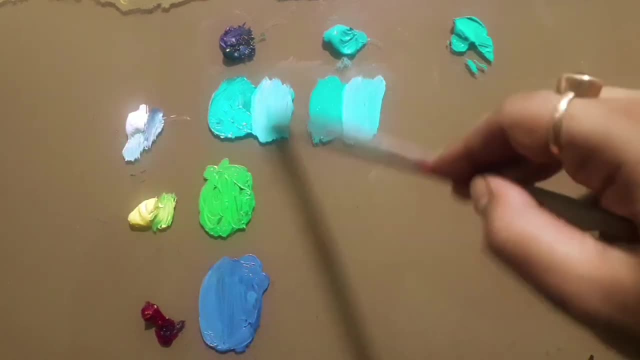 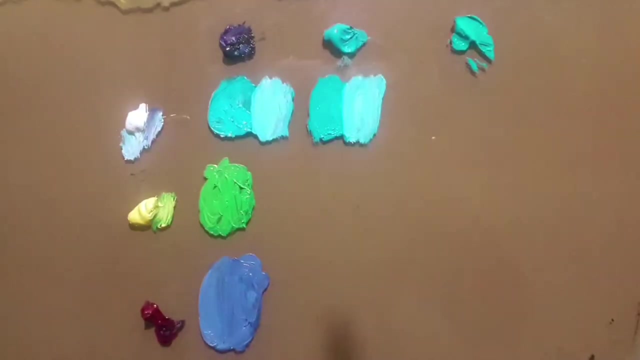 So why not add a little bit more white here as well? Okay, So that's it. Okay, Let's get our values very close. Yeah, more or less similar. So I think this color is also Thelomade, So there is no problem with this one. 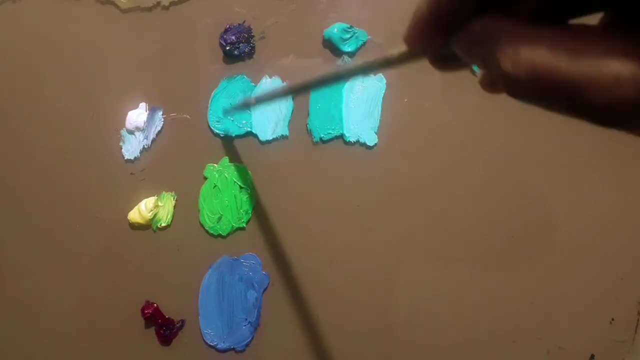 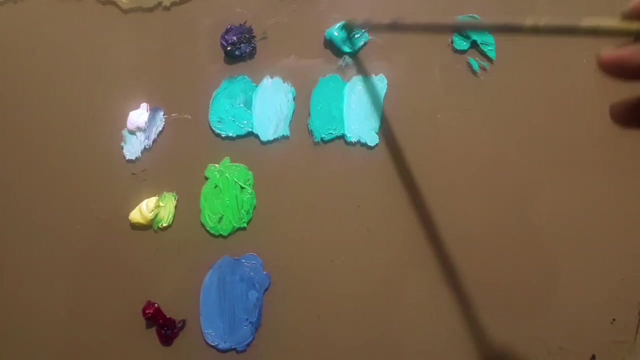 So we are practically looking at this color which is very closer to this value range, And it's a mixture of Thelo Blue and Thelo Green. Let's look at what it can do with a yellow, A yellow, A lemon yellow is a very bright yellow. 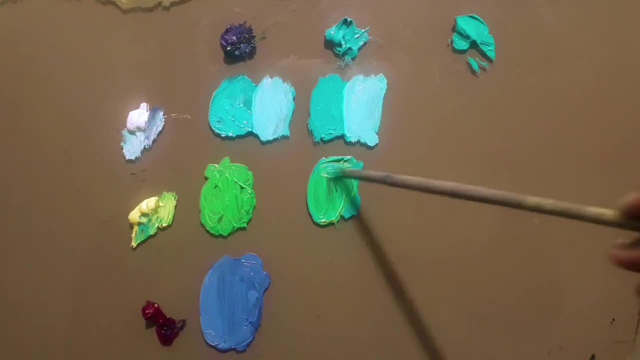 Let's see if it comes anything closer to that. One thing I'd like to mention is that this color has white added to it already, whereas this mixture does not have any white in it. It's just pure Thelo. Pure, you know, Thelomade. 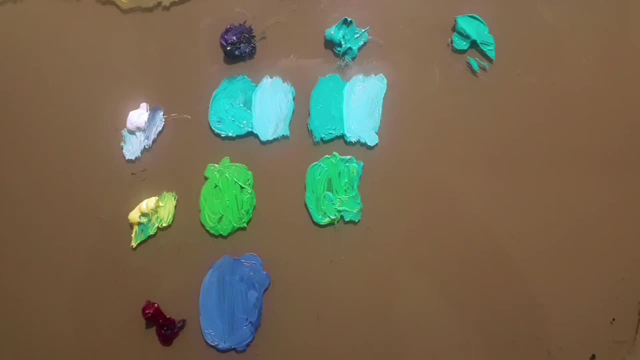 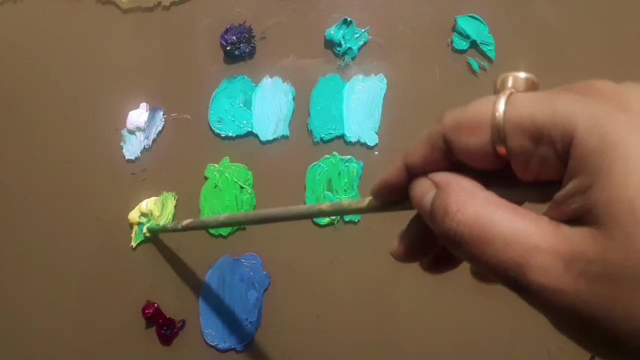 Okay, It's a mixture of, you know, Thelo Green and Thelo Blue, So all the colors that you see are a mixture of three pure colors, whereas here there's an element of white, So it may require a lot of yellow to make something like this. 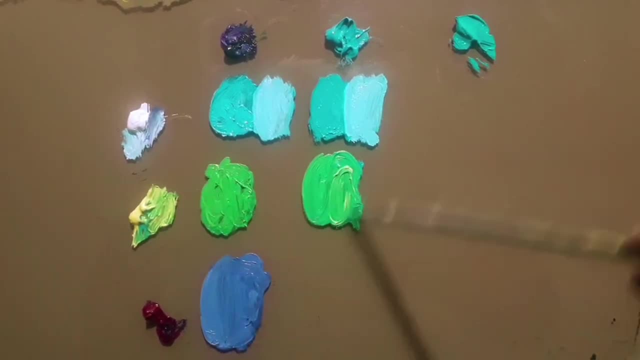 So this is one kind of a downside of using this kind of a color. Okay, So I can see that the white mixed into this color. Okay, So I can see that the white mixed into this color is creating some sort of a hassle in. 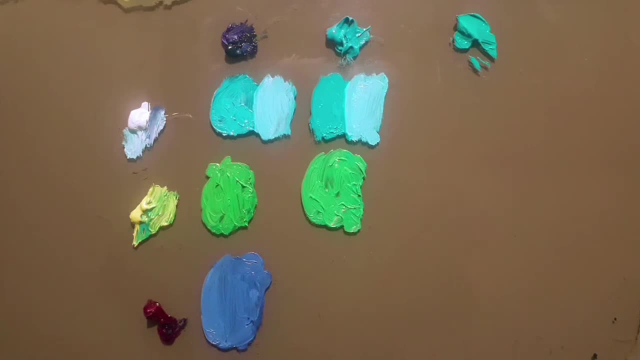 producing a true green. Let's just add a little bit more yellow and take it to the warmth level of this color And let's see what it does to the mixture. So it needs a lot of- you know- yellow to get to something like this: a very bright. 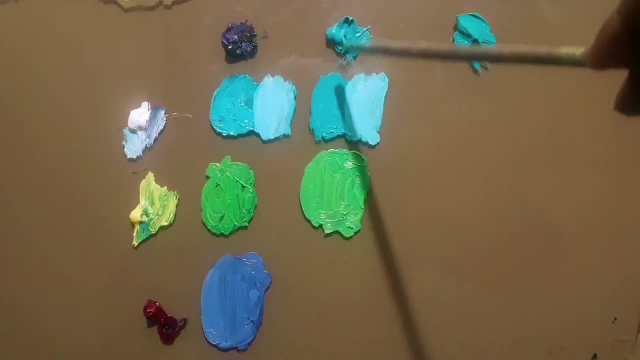 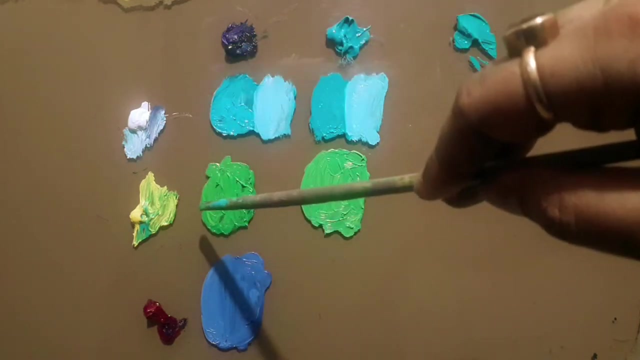 green, So the effects are not similar. You can get better results with this. This is a mixture of a mixture, and this is a mixed turquoise and this is a mixed green. This is a mixed blue, but the results are stunning with this, rather than this one, which 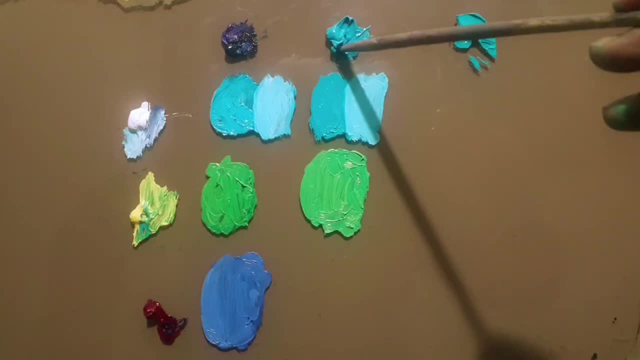 is slightly more cumbersome. Let's mix blue with this, And I think the same problem might appear due to the mixture of a white into this color. So one thing I'd like to point out: that when you'll be using this color, you would be using 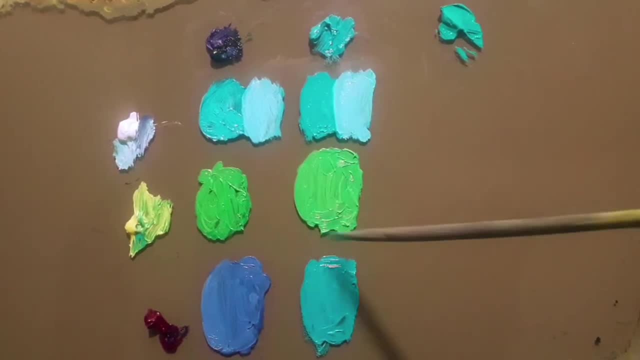 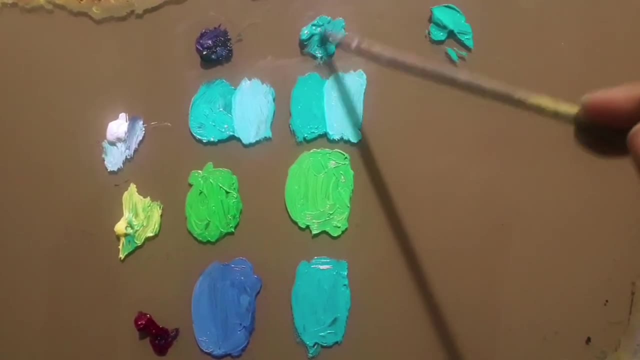 it for achieving a good cyan rather than a good mixture of you know blue. Okay, So this is a mixture of you know green or a blue. It's mostly the purpose is using a cyan color, So on its own this is absolutely perfect. 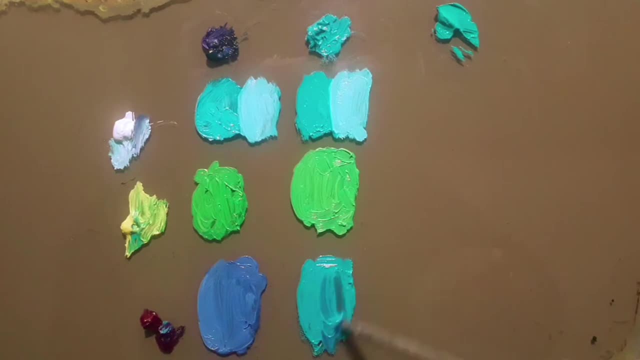 But let's test the capabilities. I am hoping that, since you know, titanium dioxide itself has some blue bias, it may not become a problem, or too much of a problem, to create a good mixture, To create a good blue with this mixture. 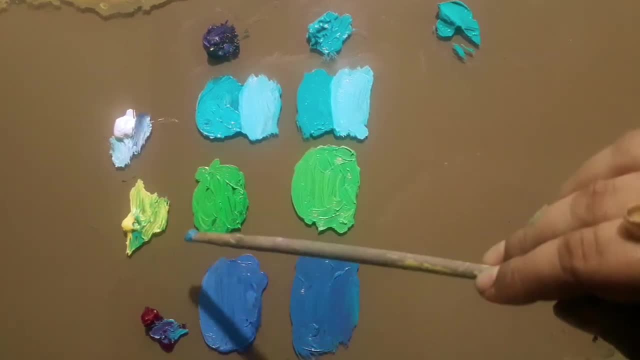 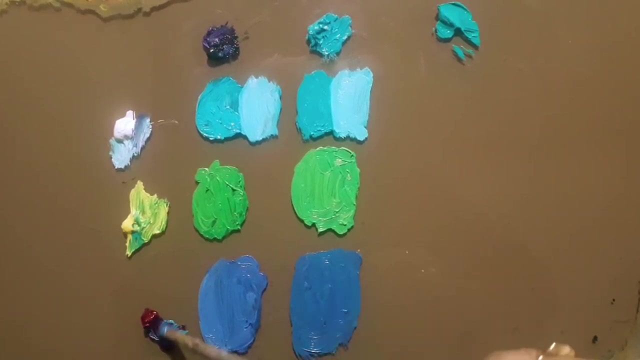 One thing I'm hoping: that, since this you know color already has a white and titanium white in itself has a blue bias to it, it may not be a big problem here in achieving a blue And as you can see that I'm achieving a quite a good quality blue, although may not be similar. 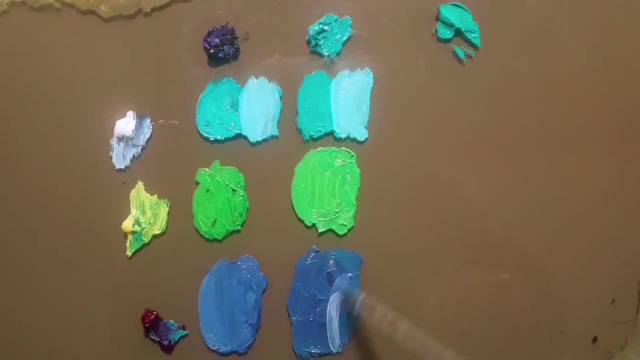 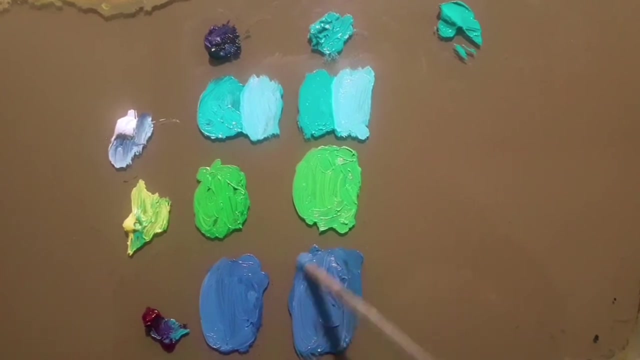 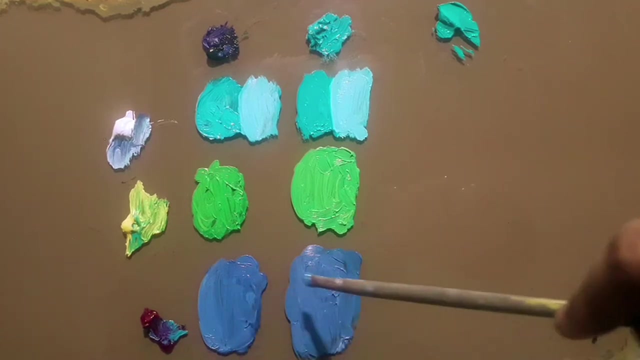 to this. Let's just tint it a little And make it Blend it into something like this: Well, not a big problem. I mean, results are more or less similar. Here it's a little bit more purer because of the presence of a Taylor blue. 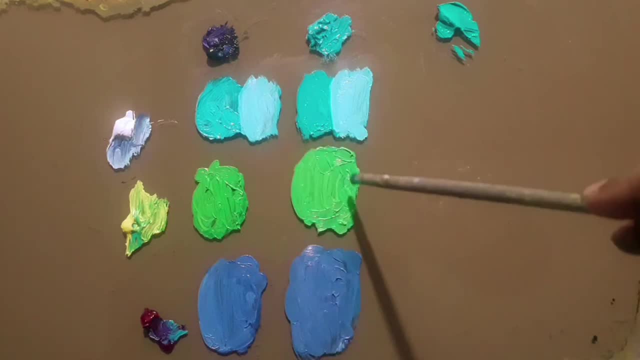 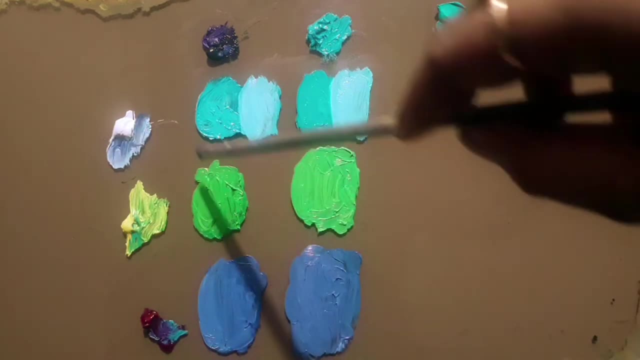 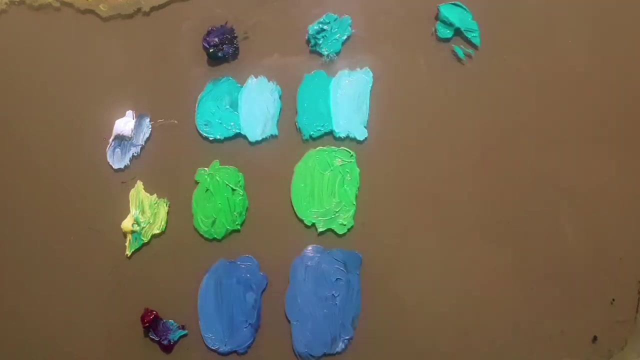 So there is no problem. Only problem that I have found is here, But that is not much of a problem, because you'll be adding more yellow to this color to achieve a good quality brightness. Otherwise, all of these colors look pretty similar. So Taylor green and Taylor blue mixture and the mixture of Taylor blue, Taylor green and 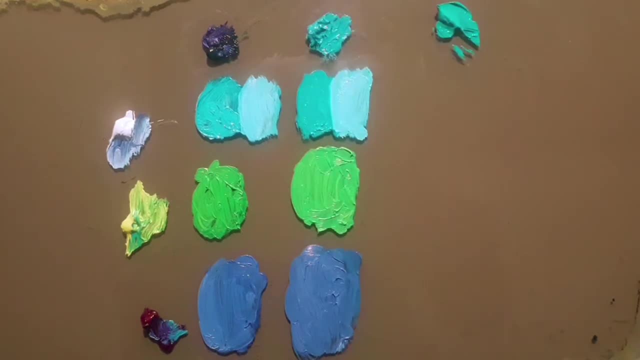 white, They do not look very different. Now here is the big area where we will test, and this is a very popular color nowadays. I consider this as the color of this century, perhaps because you know people are talking about turquoise, cyan, blue, green, aqua, blue. 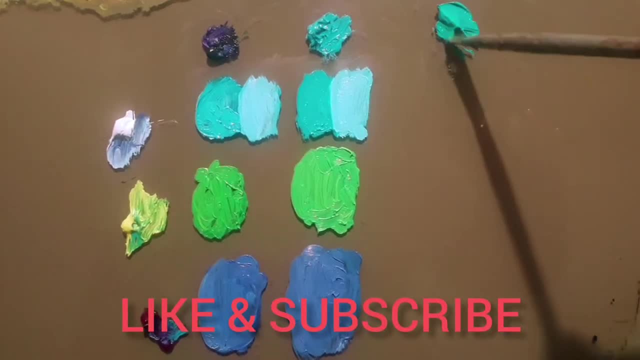 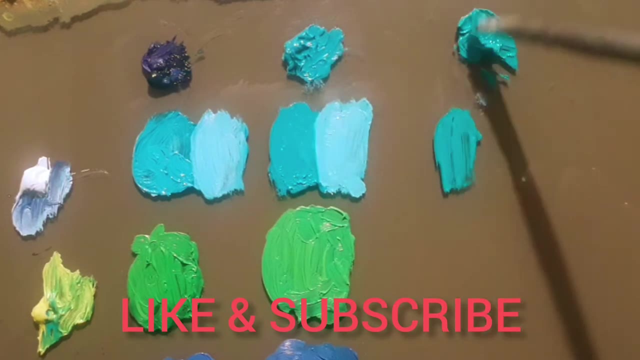 I don't know. They're just fucking talking about turquoise all the time. So let's just test this. pure colors capabilities. Overall, we can see in mass tone that it already is more powerful than a Taylor mix At all levels. This is brighter than all of these two. 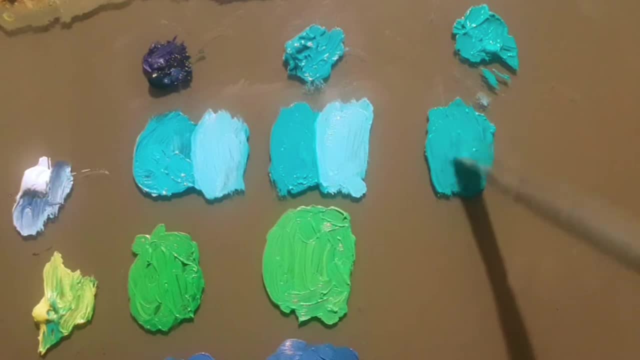 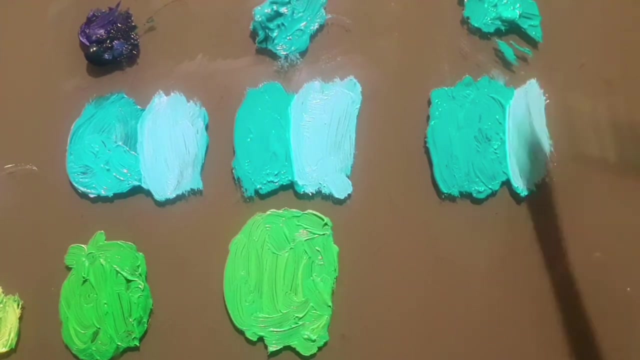 And since this is a single pigment color, I'm hoping that this might result into brighter mixes. Okay, hmm, this looks amazing. now let's add a little bit of white to this color and let's see. what does it produce. it is a mineral color, so there might be a chance. 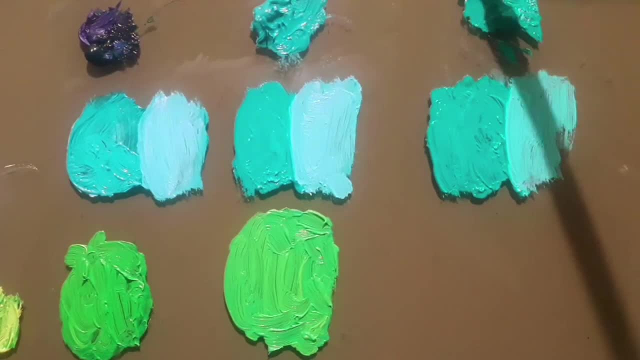 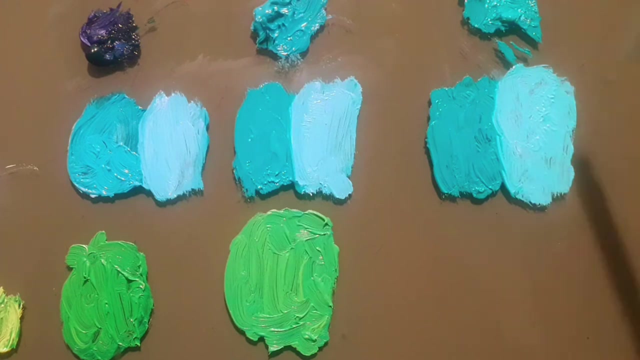 that it becomes very similar to this, but I'm trying to understand what is the value of having this color. we are closer to this value range. it's looking quite similar. so overall, you know, although this is a very pale color compared to, you know, the mastone, it looks very similar, except for that. 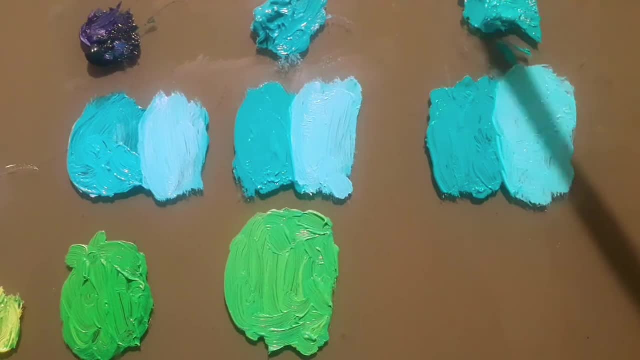 this color has a little bit more of the tone of the pure color and these are, like, slightly more greish in nature. so you know, even the brightest or the palest tones actually have a colorMAN color. overall, Lash fight is a very is has more color into this, so, which is a good thing. and now let's test the pure. 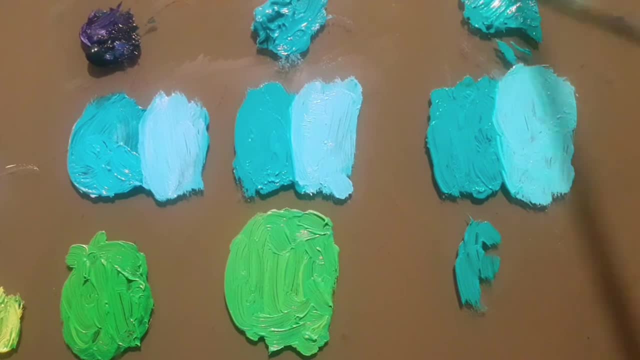 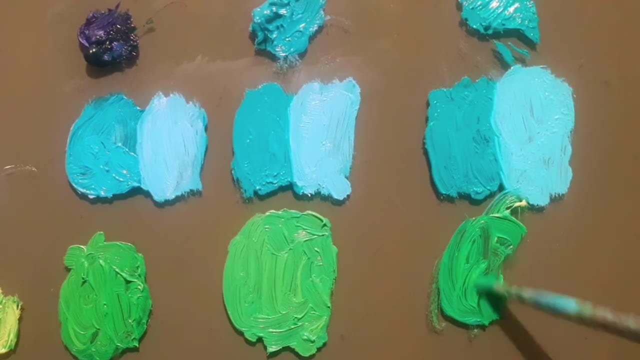 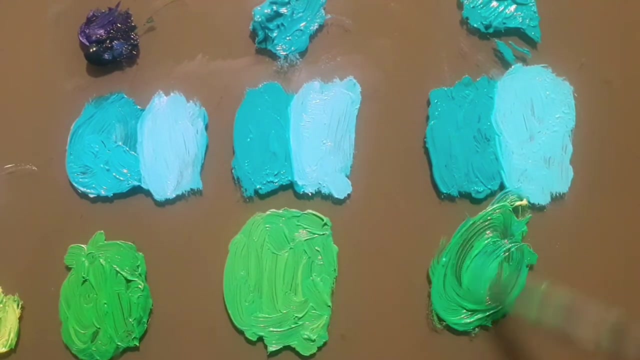 color here with a little bit of yellow. it's better to mix slowly rather than too much. let's just add a little little by little. I'm adding almost all of the lemon yellow that is left, and let's see. what does it mean? well, the result, the mixture, is very similar to telomix. even here it's. 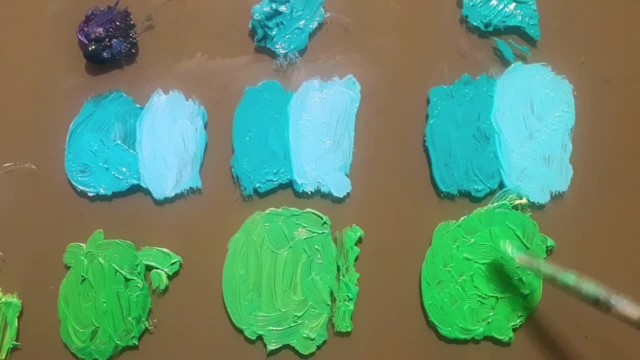 unnoticeable. it's actually very similar in nature and practically there is no difference. maybe this one has more similarities with this one, but this might be a little dull because of the presence of this white, whereas you know, these two telomix are very similar in nature and cobalt teal mixed with yellow. they look quite. 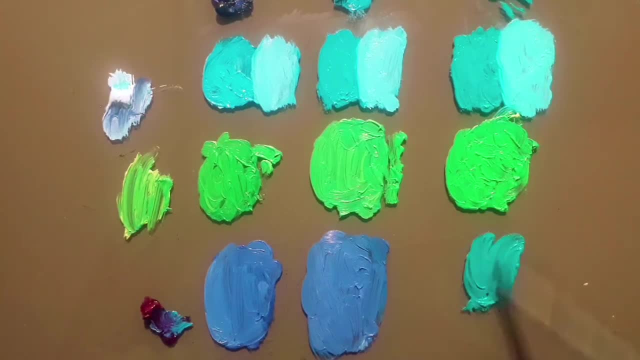 similar. now let's look at this: what it produces with a little bit of magenta. well, the, I think here it produces a very good result and very vibrant. let's just continue to mix. well, the, I think here it produces a very good result and very vibrant. let's just continue to mix. 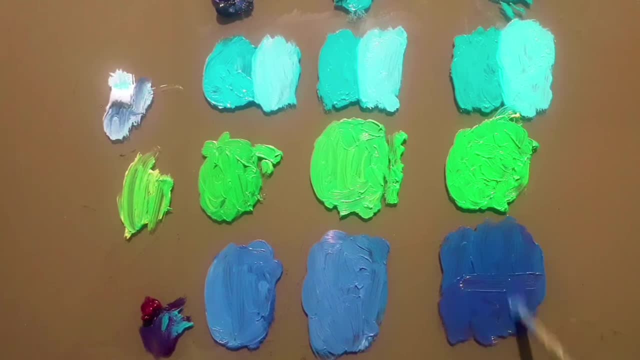 well the I think here it produces a very good result and very vibrant. let's just continue to mix this magenta into ritual. this is a very- you know- beautiful blue, smoky and very useful and more vibrant than these two mixes probably may not have. you know the brightness of this blue, but still it is exceptional one. 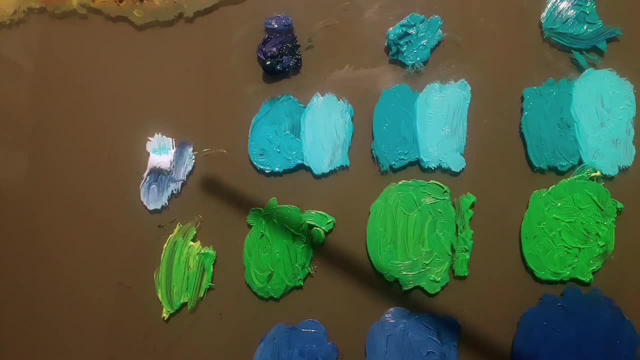 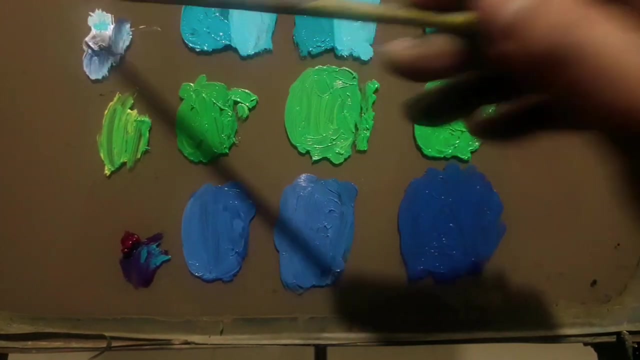 cannot be compared against a real blue pigment. for instance, there is a thaler blue. this is all of. this is, most of the time, will be, uh, you know, smoky kind of a blue, slightly gray, slightly duller, but this is actually a blue. now let's check the. what happens if we mix a little bit of white? 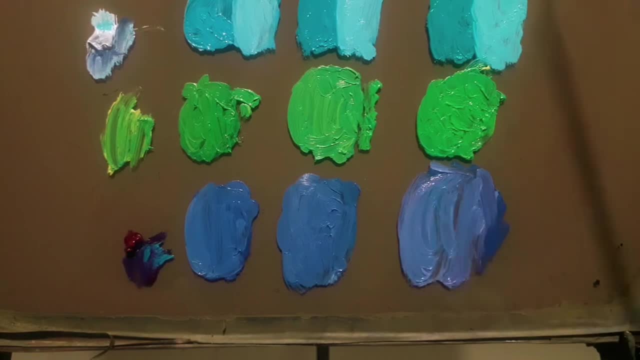 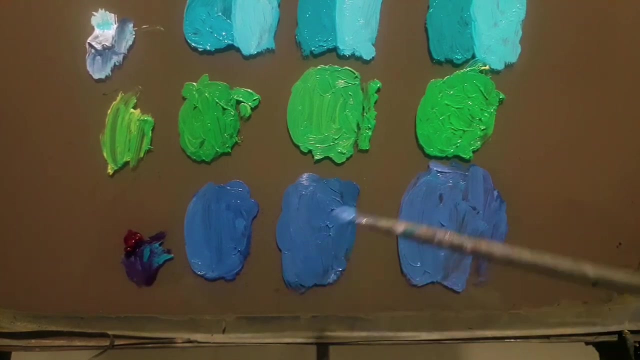 it has turned violet. so i'm going to add a bit more cobalt teal here, but more teal meaning going towards green side rather than blue side. maybe a slight amount of magenta. are we close slightly brighter? slightly, put more magenta here, okay, so what i can see is that this mixture here. 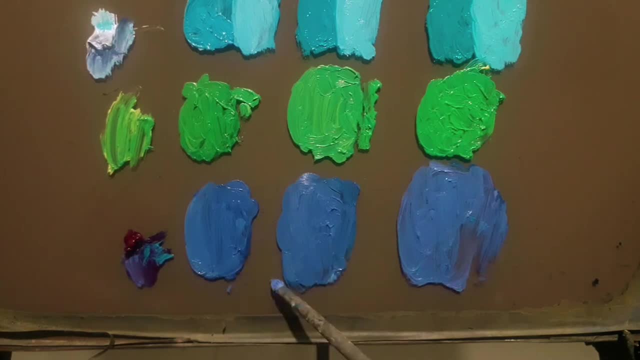 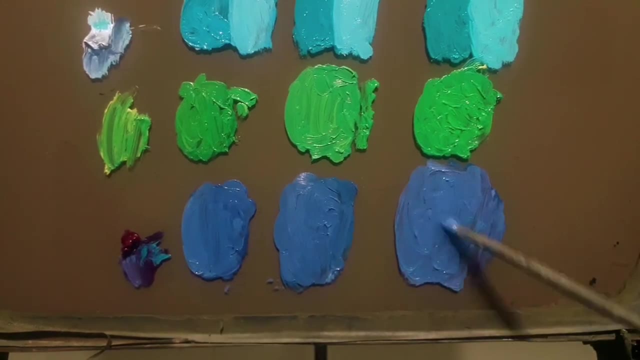 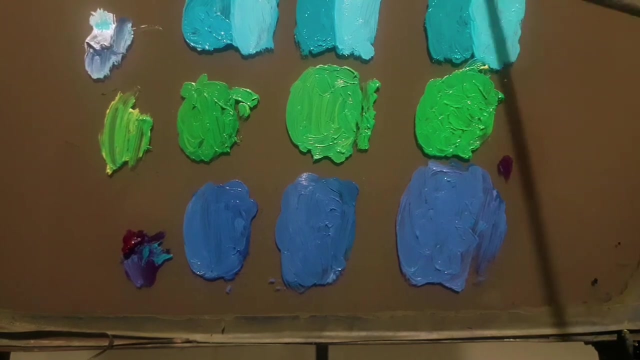 is the key differentiator, because these two are looking pretty dull, although the mixture above, without the white, that will be quite natural. and here we are getting a more colorful mix and we have added white and let's just mix a little bit of teal here and it produces a beautiful violet color. let's just add a little bit more teal. 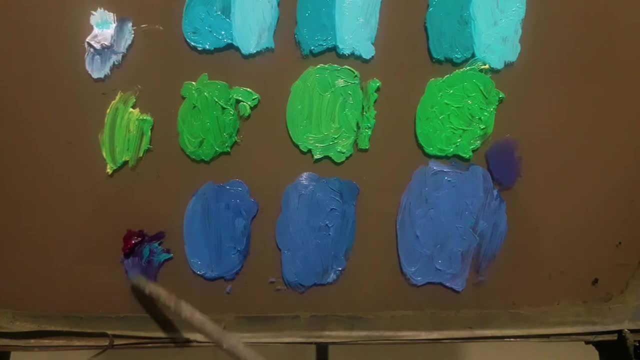 we are getting this smoky bluishness, but the violets are extremely pure, no doubt about it. it's not inky dark. this has comparatively a lighter value, violet, but very beautiful, very pure. maybe through camera it's not that apparent, but if i continue to add violet or the purple here, you can make a guess. so overall, 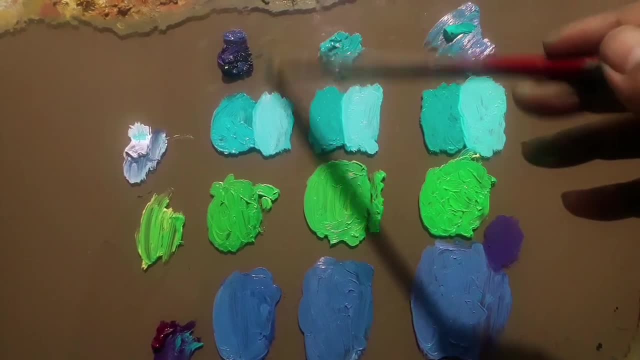 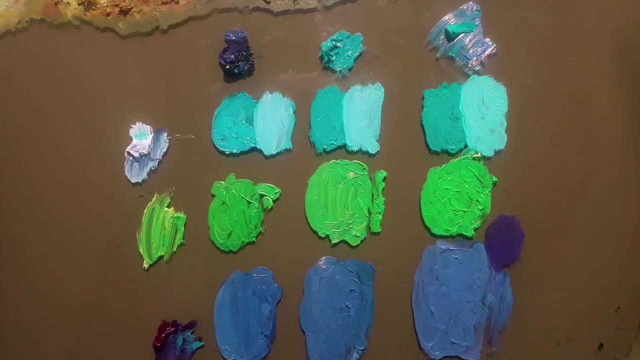 looking at all of these, you can quite clearly see that the phthalo colors are still retained here, because phthalo colors are industrial colors, they are organic pigments and- uh, you know modern developments. so they are very powerful and, uh, you know, slight amount goes a long way. 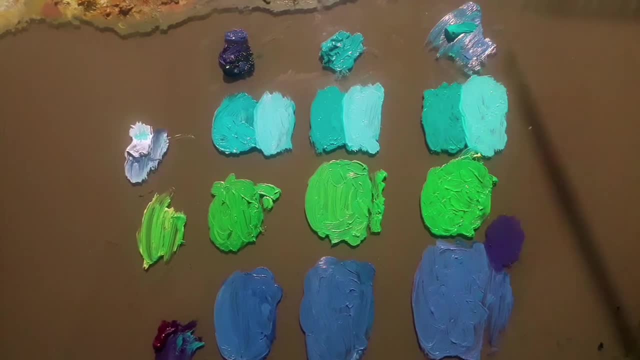 whereas this is a mineral color, so it takes a little time, you know you can see that. uh, you know, while matching of these colors it has. you know, i have used up all the all the cobalt, but you know you need to use a little bit more. 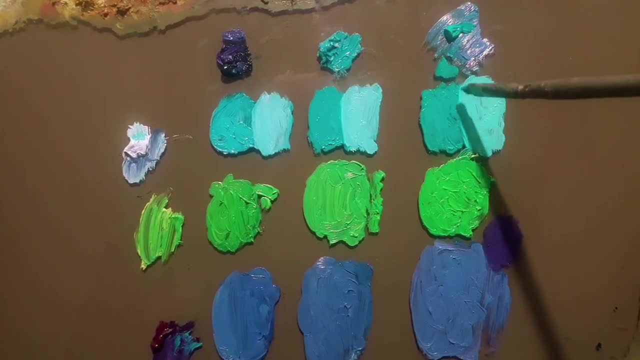 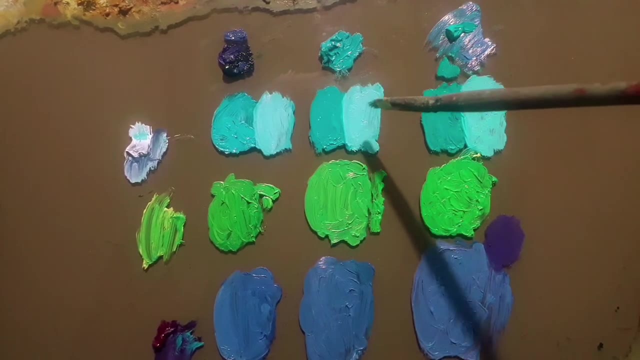 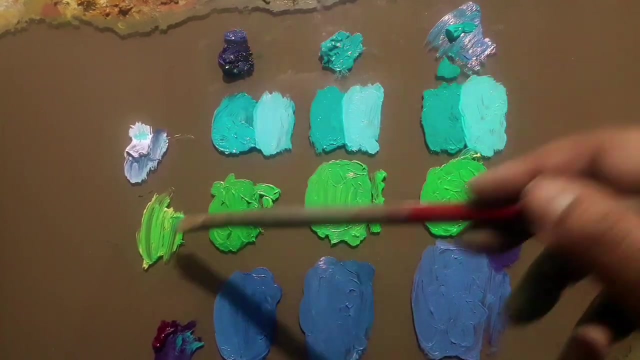 and the results are quite similar, except for this white mixture where i can see that it's slightly bit more colorful than these two and these are slightly a bit more grayish. and you know, mixing yellow, the pure phthalo and pure phthalo mix, pure phthalo blue, pure phthalo green with lemon yellow. 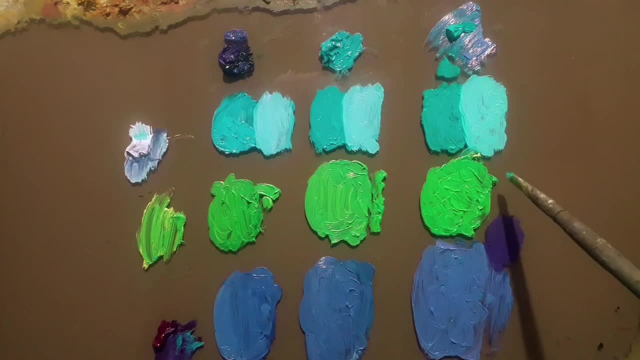 produces a good result, very similar to. you know the result that was mixed uh with the cobalt teal and the lemon yellow, so there is not much difference here and here and in terms of the mixing the blues, i think this has produced a better result. as well as this, 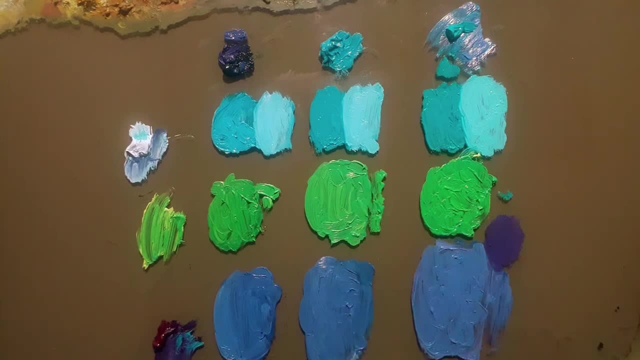 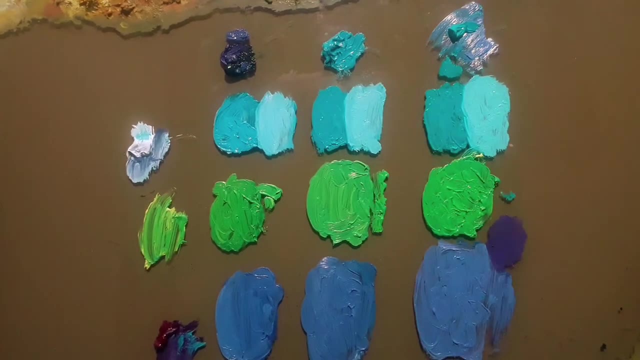 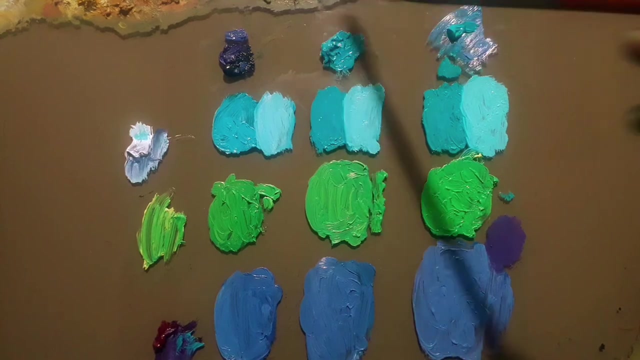 this one, and proprietary mixture is not that effective- maybe slight bit, so you know. my conclusion is that if you want to get a good turquoise at a lower rate, i think it's better that you get this color, because this is just one color. you don't need to invest in two colors plus. 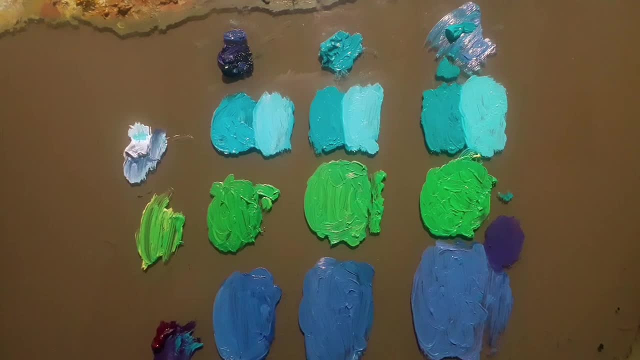 using up white and it's totally about using the turquoise and not for producing a green or a violet or a blue. it's for this particular color, so this will do its job. when you add a little bit of yellow, it will become a bit more warm. if you need a little bit more bluishness, you add a little bit of purple. 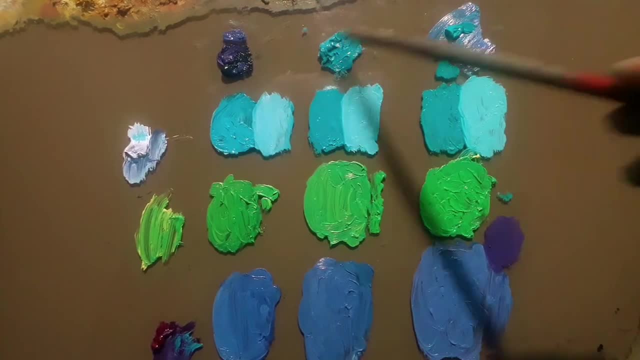 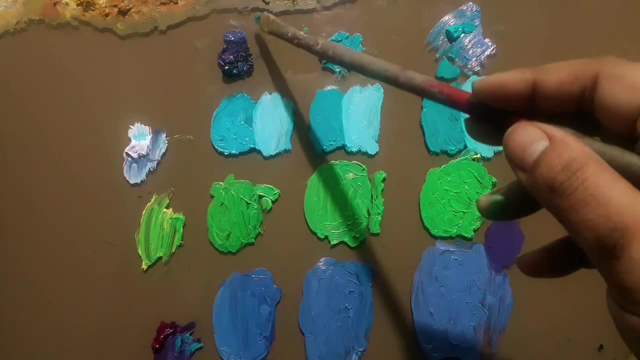 or magenta, so it will become a little bit more blue. when you add white, it will become a brighter color. layer upon layer, this will become a brighter color. similar results can be made in the same way can be achieved with the, the telomixes, pure telomixes, with white or yellow or magenta, but this color 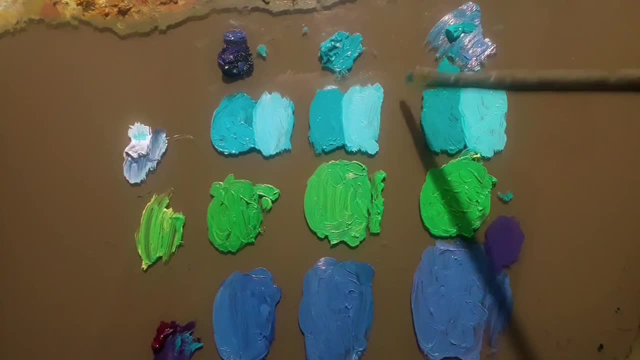 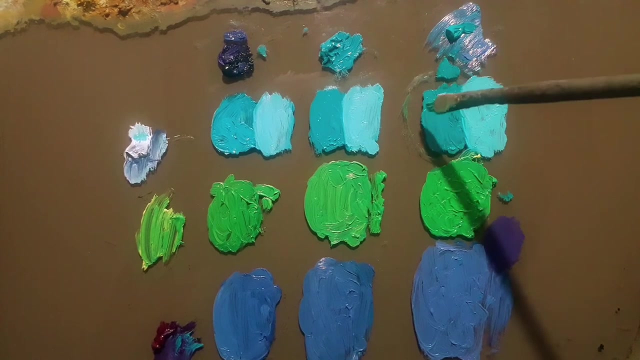 on its own is a pure color, and if you- uh, if you can buy this one- and since this is a very expensive one, you need to think twice before buying this one. but if you can acquire this color, this has no comparison. and these are mixed colors and this is a pure color and this has its- you know- own kind. 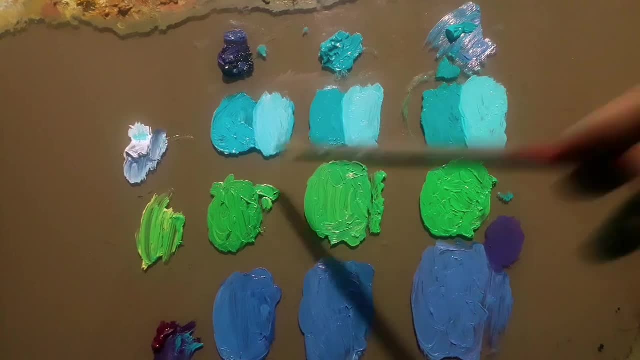 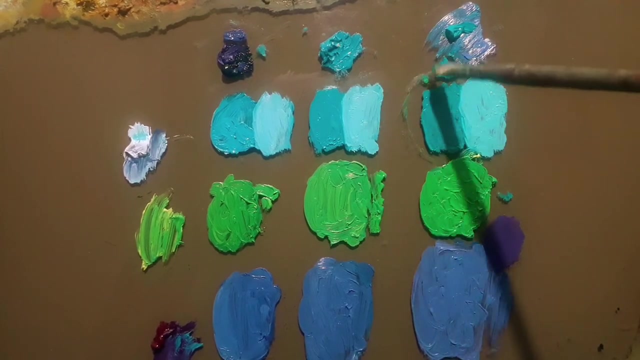 of a luminosity and brightness that you know these colors cannot mix. already they are showing that they have white mixed into it and this is this doesn't have any white. this is a pure, you know, turquoise color and overall this is the brightest turquoise color in the market. so you know, very useful and when you're.